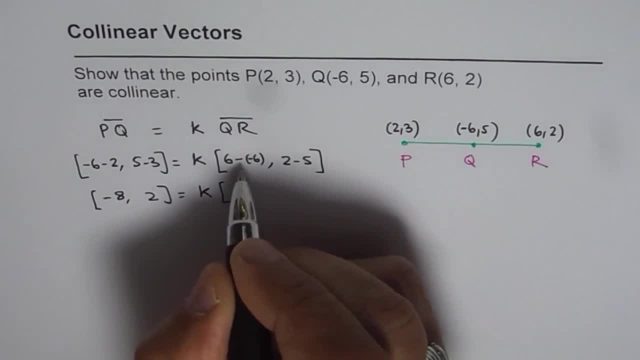 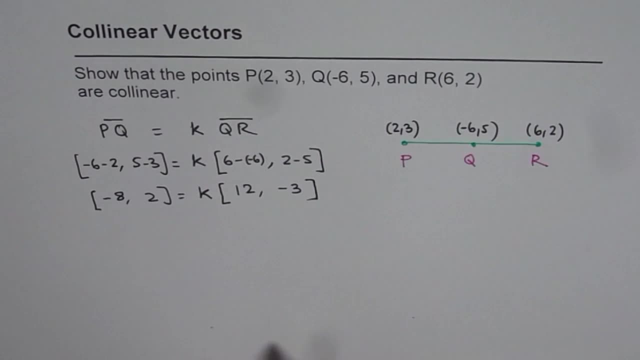 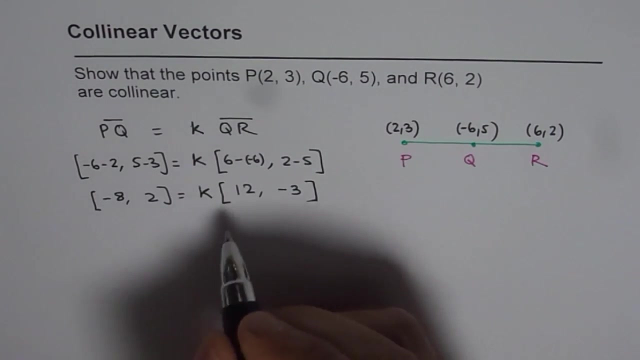 2, equals to K times. here we have 12, minus 3.. Now we have to figure out if there is a value of K which can satisfy this equation. So if we compare the x values, that is to say that minus 8 equals to K times 12.. So that gives. 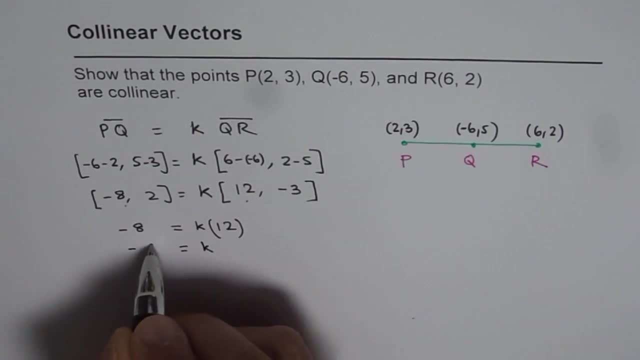 you the K value of minus 8 over 12.- So that means K is equal to both- can be divided by 4, so we get minus 4 times 2, 4 times 2 over 3. So K is 2 over 3.. Now, if 2 over 3 is equal, 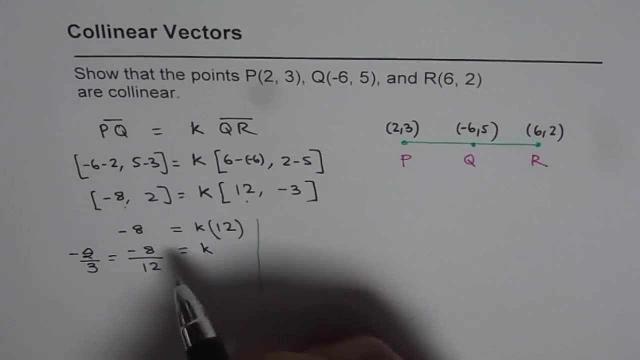 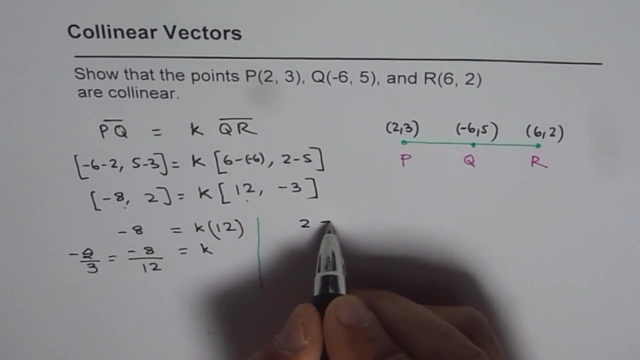 works for the y value, then we say, well, it is perfectly fine. Or the other way is, we can equate: the second part, which is 2 equals to minus 3k. Now from here we can find what k is From k. 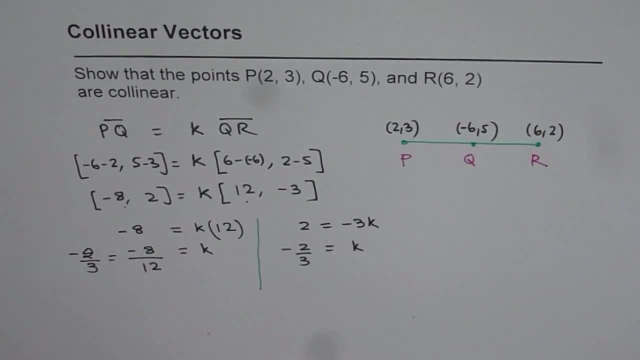 will be minus 2 over 3.. Now, since we get the same value of k, which is minus 2 over 3, we can write from here: right? So from here, since we get k as minus 2 over 3,, so from here. 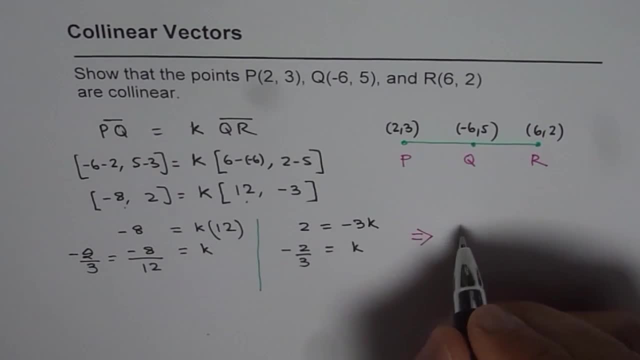 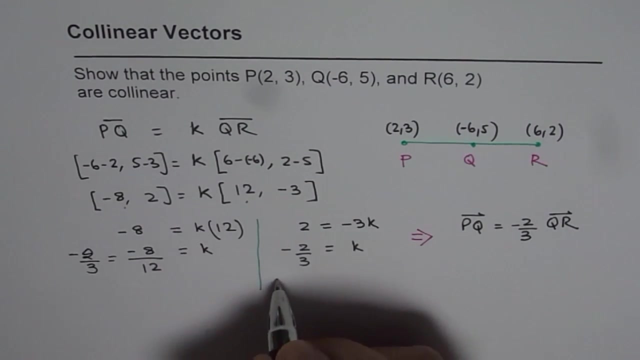 we can say that pq is equal to minus 2 over 3. qr. Correct. Since k is minus 2 over 3, I could have written this equation as: minus 8, 2 equals to k, which is. let me write now: 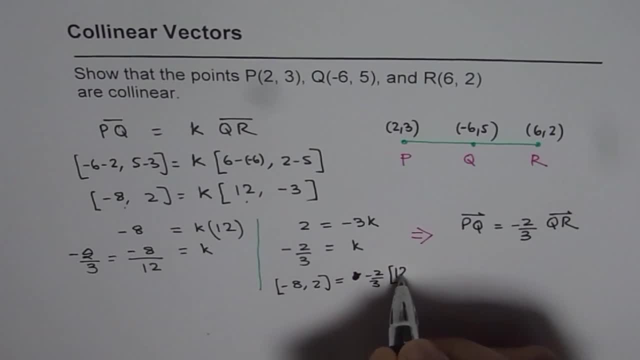 minus 2 over 3, right Times: 12 minus 3, correct. So then we will get the same as k as minus 2 over 3 qr, which is minus 2 over 3 qr, right. So then we will get the same as k as minus 2 over 3 qr. right Times: 12 minus 3, correct. 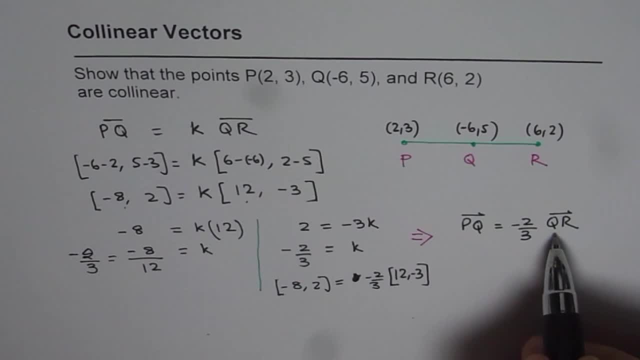 That implies that pq equals to minus 2 over 3 of qr And therefore they are collinear Scalar multiple. do you see that? So that is how you can show whether the given points are collinear or not, right? So given points are collinear if they lie on the same line, correct?